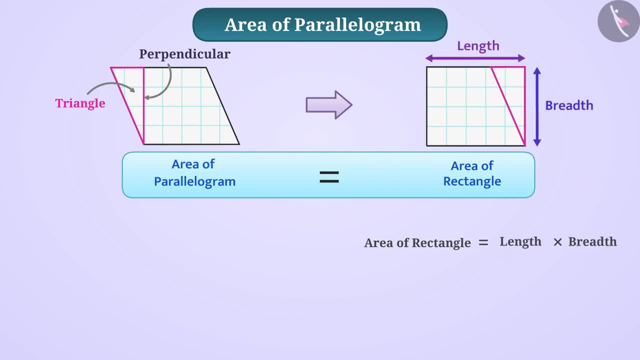 So we have to make the area of rectangle equal to area of rectangle. So we have to make the area of rectangle equal to length multiplied by breadth. Here length of rectangle is equal to length of base of parallelogram. The line on which perpendicular is made will be considered as base of the. 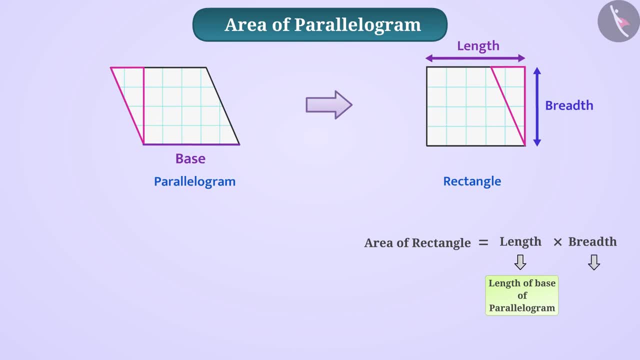 parallelogram. Similarly, breadth of rectangle is equal to height of parallelogram, which is the length of the perpendicular. Therefore, we can say that area of parallelogram is equal to length of base of parallelogram multiplied by height of parallelogram, or area of parallelogram is equal to base. 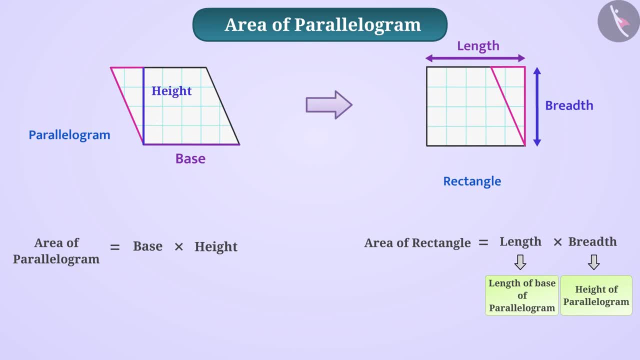 multiplied by height. if we consider length of base of parallelogram as B and height of parallelogram as H, then we can write: area of parallelogram is equal to Base multiplied by height. With the help of this formula, we can easily find out the area of parallelogram. 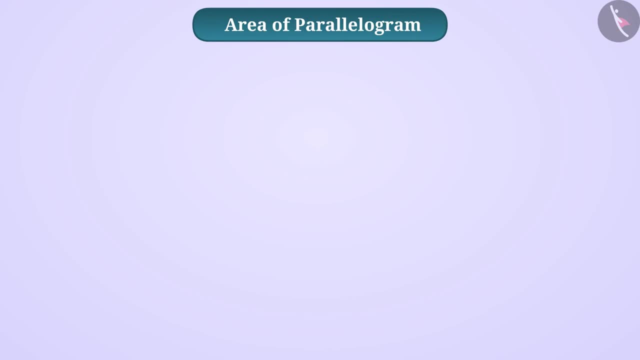 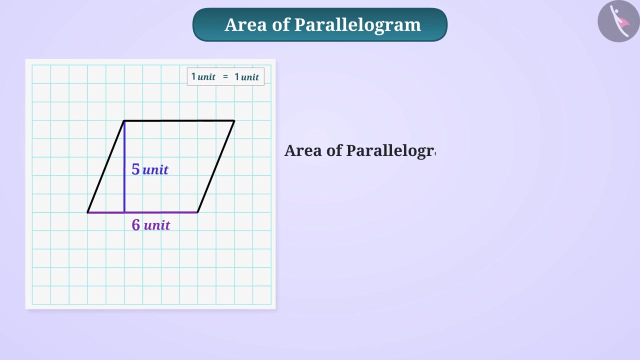 Let's find out the area of parallelogram shown Here. length of base of parallelogram is 6 unit And height of parallelogram is 5 unit. Therefore, area of this parallelogram will be 6 unit. multiplied by 5 unit is equal to 30 square unit. 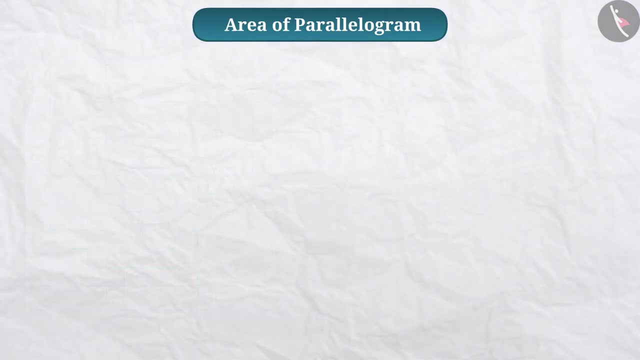 Remember that in parallelogram we can consider any side as its base. The length of the side which we consider as base will be the length of the parallelogram. On this side, the length of the perpendicular from the opposite vertex is called as the height of the parallelogram. 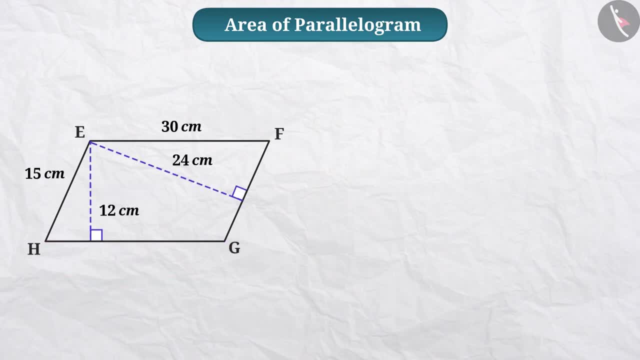 Like in parallelogram On side HG, perpendicular ED is drawn from the opposite vertex E. If we consider side HG of parallelogram EFGH as base and perpendicular ED as height, Then we get area of parallelogram as 15 cm. Similarly we also see that in parallelogram EFGH.